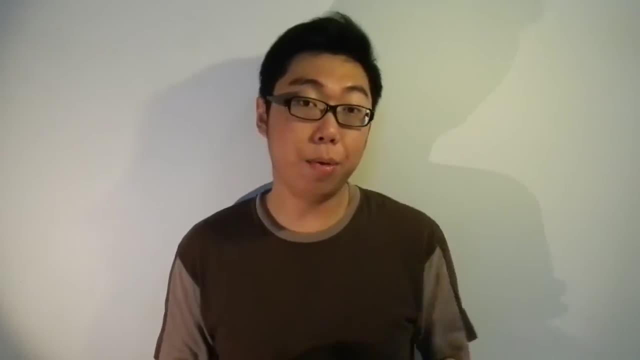 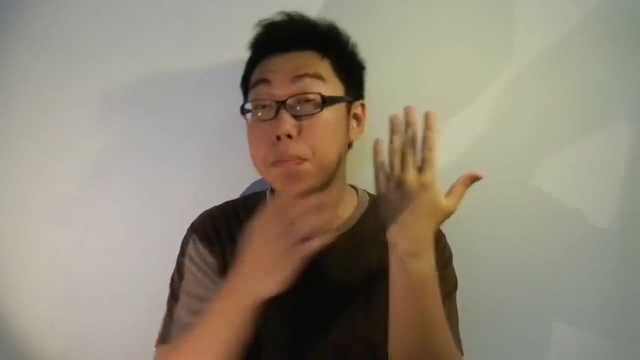 part in just playing back videos with predicted frames, And the reason for that is because, well, a whole lot of frames actually depend on this one iframe, because they just keep building on top of whatever this iframe sits. And that's why it's called a bidirectional iframe, because it's a 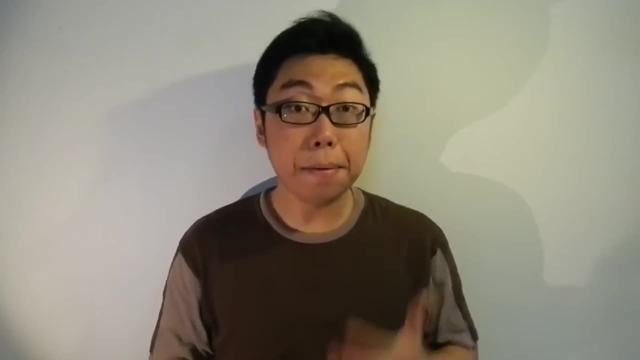 bidirectional frame, And that is why one particular factor always comes into play, and that is how far you space apart your iframes. Now, if you actually do video work, you will see your encoder have an option called GOP. What is GOP and what does it mean? 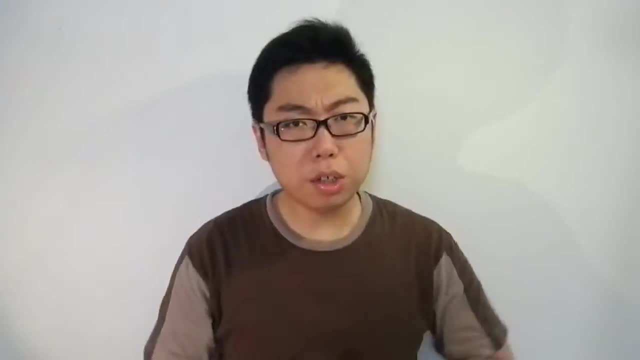 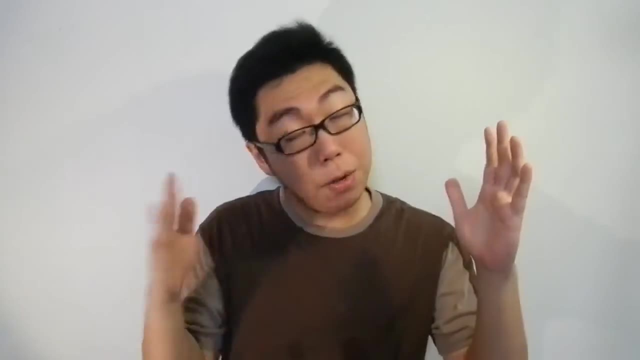 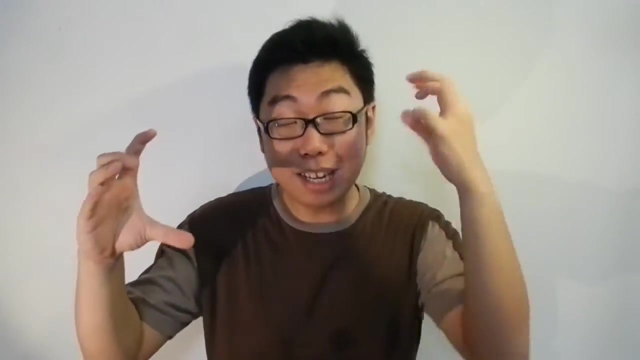 GOP stands for a group of pictures. So how do we group pictures together? Well, you see, every time you have an iframe and a bunch of pframes or bframes that actually build on top of it. well, that is a group of pictures. These are related because they share the same iframe. That's why 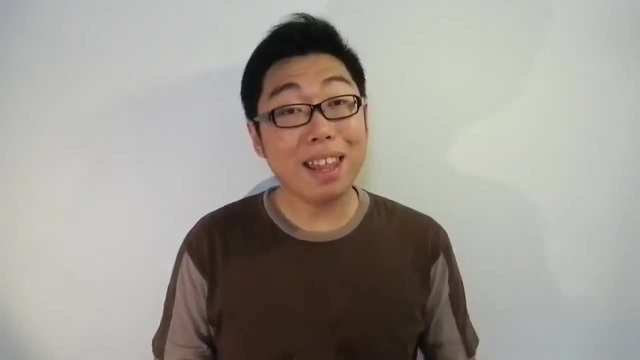 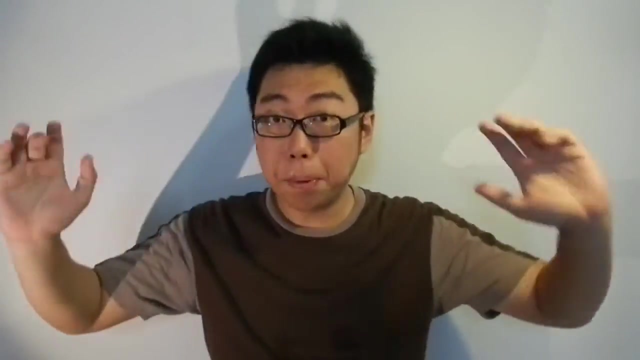 you always see the term GOP normally associated with a size, and this is exactly what the GOP option is actually affecting. So if you reduce the GOP size, essentially what you're doing is you're asking for more iframes. If you increase the GOP size, then well, because groups get bigger. 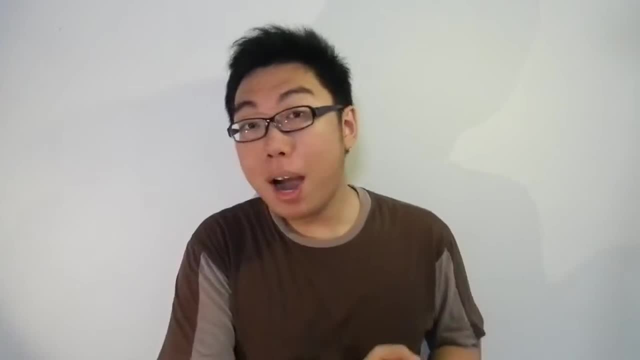 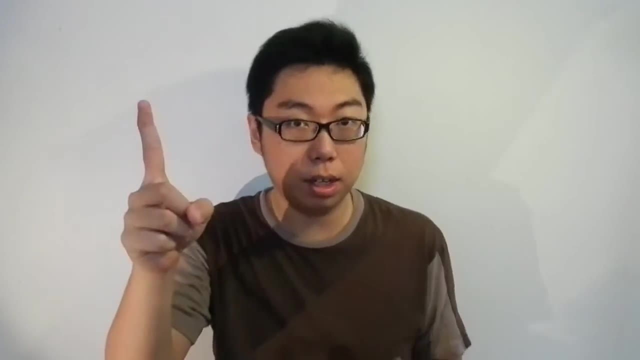 the iframes get fewer and far between. If you have more iframes, seeking and editing becomes easier because, well, you don't have to search so far every time you land on a particular frame while seeking. The downside of this, of course, is that you have a larger file size. 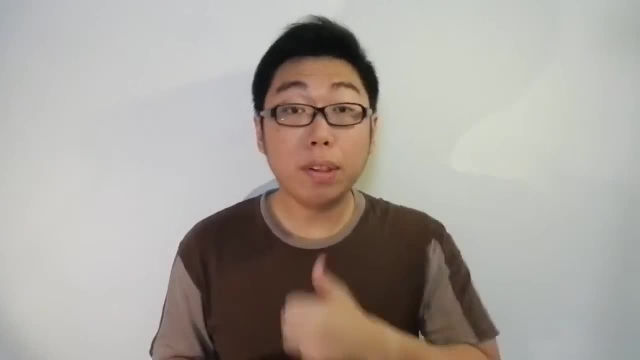 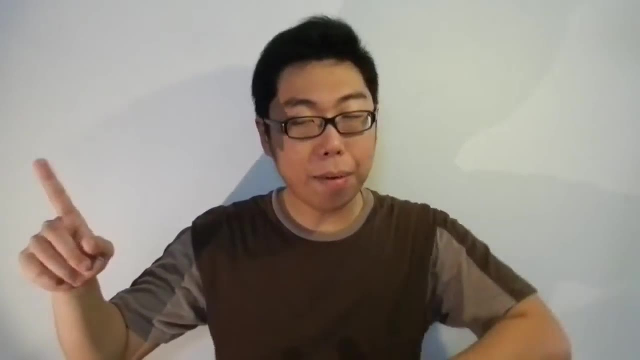 and that's because you get to throw away less information. With a large GOP, you achieve good compression, but seeking will become slower because every time you land at a frame- whatever player or editor that is actually, you know- running will actually have to go backwards and 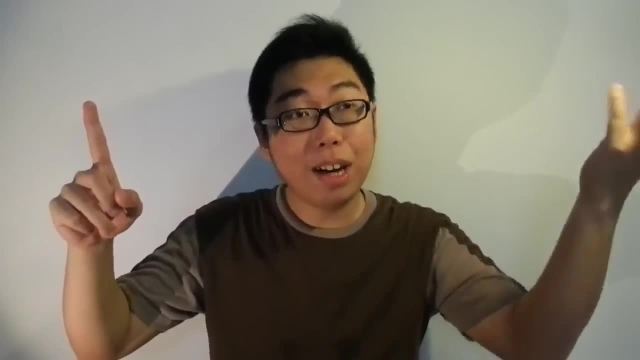 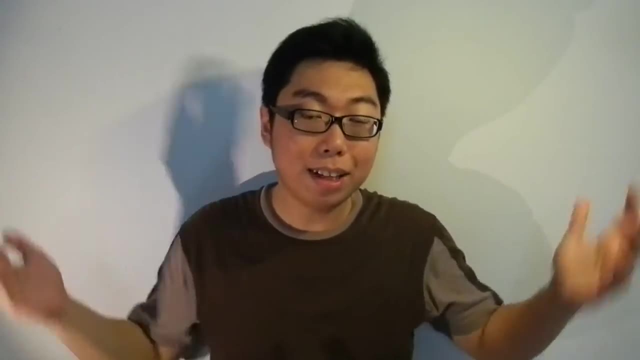 search for the closest iframe. Once it has that iframe, you're going to have to play forward through all the iframes and build up until we get to the frame you're looking for. And there you have it. that is what the term GOP refers to. 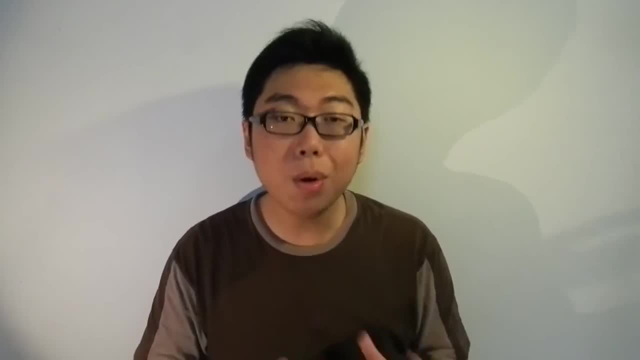 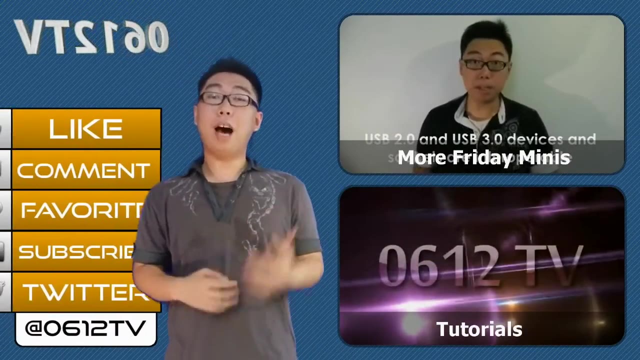 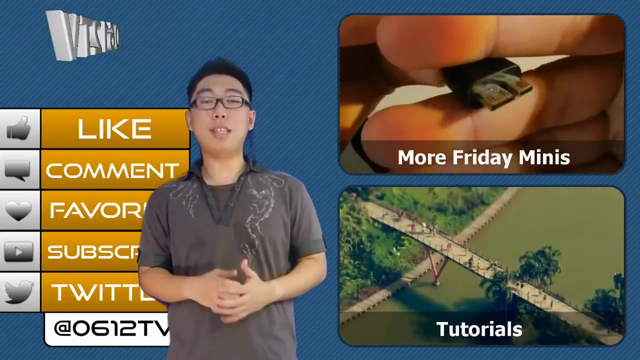 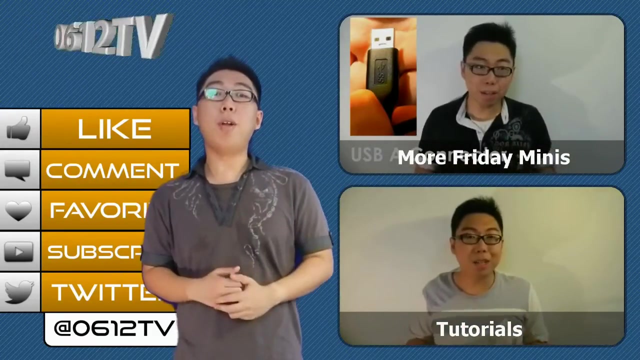 Well, I hope you learned something today. That's all there is for this episode and until next time you're watching 0612 TV And for more updates outside of YouTube, don't forget to follow me on Twitter at 0612 TV. Once again, thank you very much for watching and I'll see you guys next time.